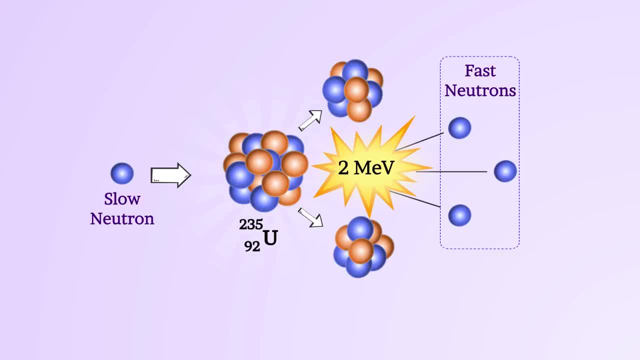 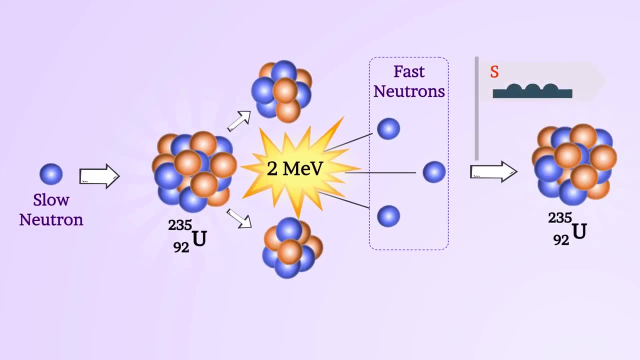 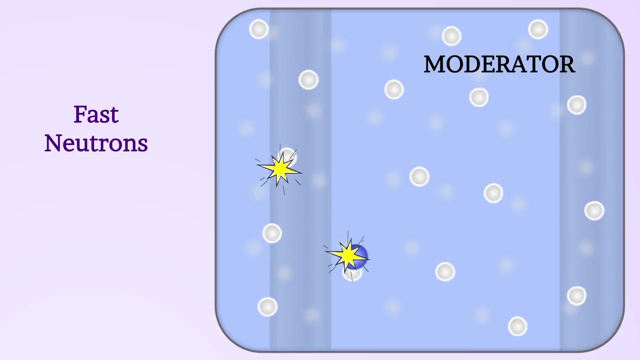 That means these are fast neutrons and therefore have less tendency to cause fission. In order to facilitate fission reaction, there is need to slow them down. The job is done by moderator by transferring the energy with elastic collision to lighter nuclei. 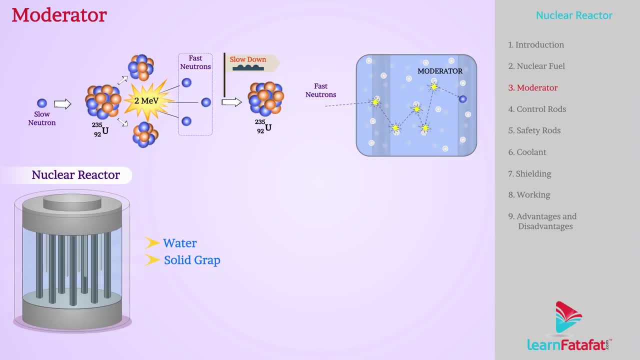 In nuclear reactors, water, solid graphite or heavy water are being used as moderators. The Apsara reactor at the Bhabha Atomic Research Centre, Mumbai, uses water as moderator. Other reactors in India uses heavy water as moderator. In nuclear reactors, water, solid graphite or heavy water are being used as moderators. 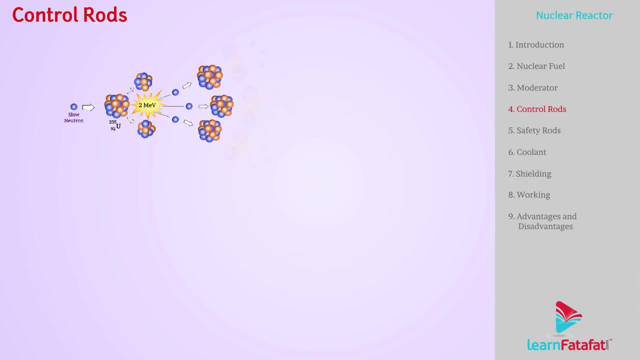 Nuclear reaction, if not controlled, may lead to explosion. The catastrophe happened in the Khaldobyl reactor in Ukraine in the year 1986, remind us the necessity of having control on the nuclear fission reaction. Multiplication factor K help us to determine if the reaction is in control or not. 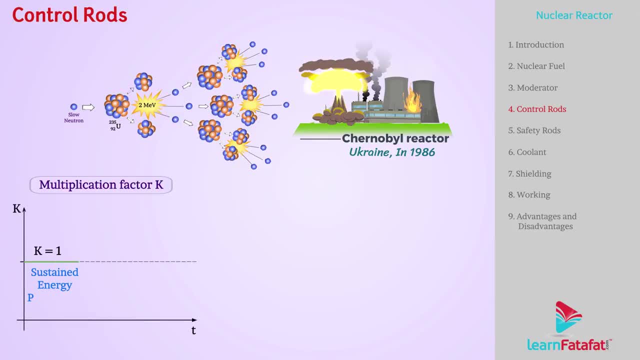 K equals to 1.0.. one is required for sustained energy production If K exceeds unity. control. rods made of boron or cadmium are inserted in the reactor core up to desirable length. The rods have ability to absorb neutrons and therefore the nuclear reaction can be controlled, thereby bringing 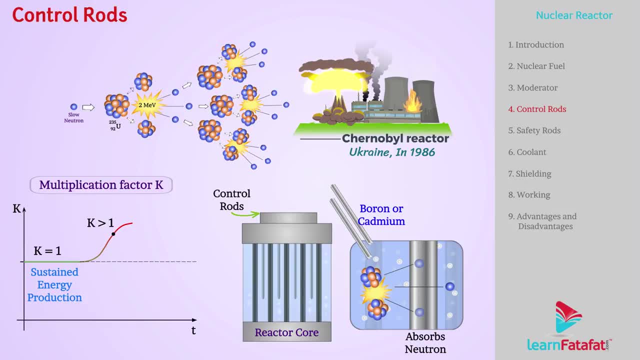 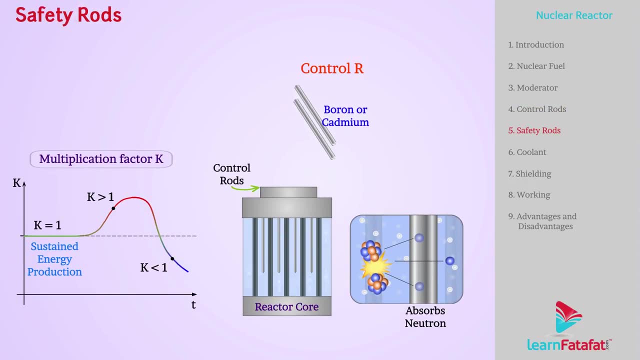 multiplication factor down unity. Safety Rods: In addition to control rods, the reactors are provided with safety rods. These rods can be inserted into reactor in order to bring the value of K below unity, thus keeping the power generation safe. Coolant Heat produced in the core is absorbed by coolant. 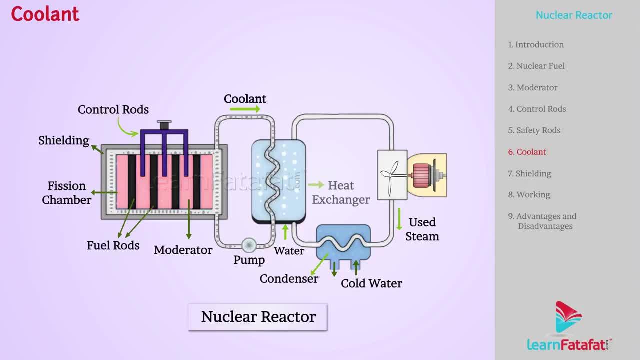 and then passes this energy to water in a heat exchanger so as to produce steam. Steam is used to drive turbine coupled with electric generator, and hence electric energy is produced. In general, for ordinary temperature range, water or heavy water is used as coolant.